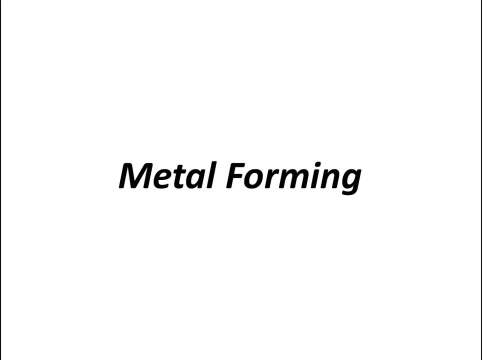 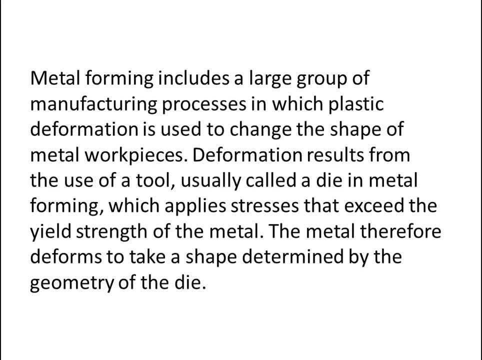 Let's talk about metal forming. Actually, metal forming includes a large group of manufacturing process in which plastic deformation is used to change the shape of metal workpiece. So in this here, actually we actually shape, change the shape of a material, and the shape is changed by plastic. 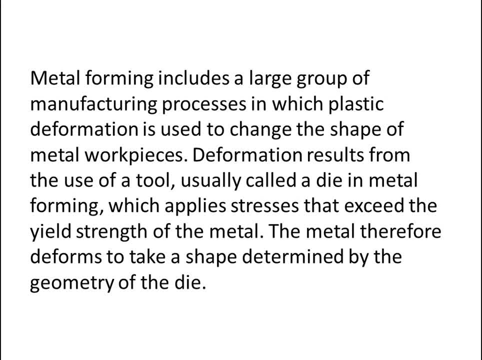 deformation. Deformation results from the use of a tool, usually called a die, in metal forming So the metal. the tool that we use here is called a die, which applies stress that exceed the strength of the material. So if you want to bring any plastic deformation, we need to exceed the 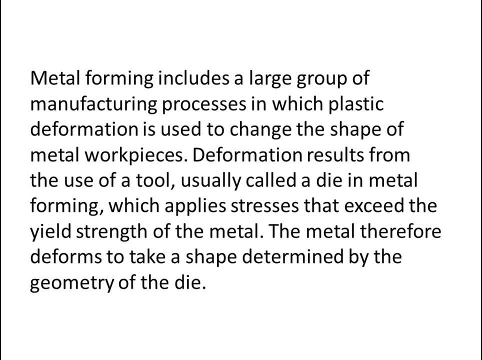 strength of a metal. The metal therefore deforms to take a shape determined by the geometry of the die. That means the deformation will not be carried out in a plastic form, but the deformation will be carried in a plastic form. So the deformation will be carried out in a plastic form. That means 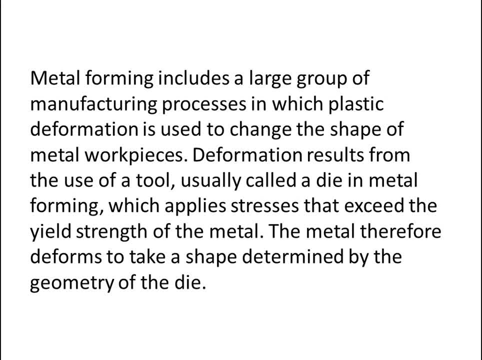 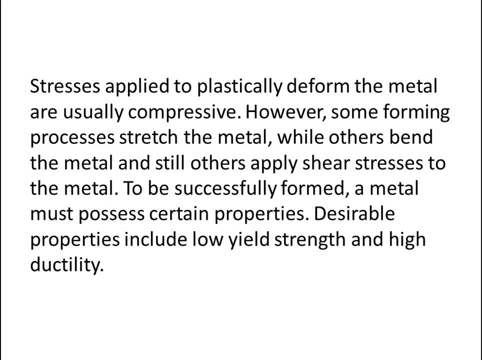 the die determines the shape of the metal. again, stresses applied to plastic deform the metal are usually compressive. so here we are: we apply the compressive stress. however, some forming processes stretch the metal, while others bend the metal. and still others others appreciate stress to the metal. so some 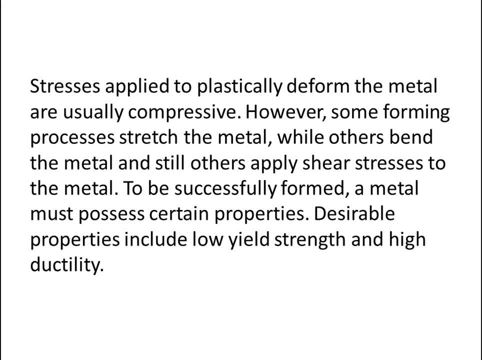 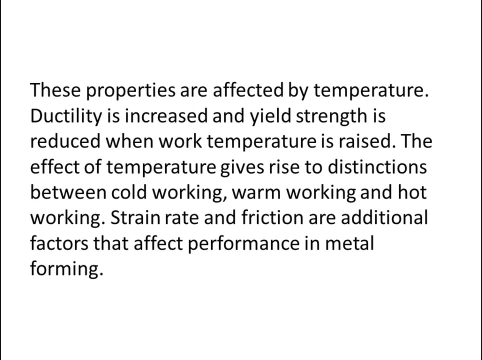 forces are stress stretched and some are bending, and forces are bent and some forces are shear stress. now, to be successfully formed, a metal must possess certain properties, and the properties are low strength and high ductility. okay, these properties are affected by temperature. that means ductility is. 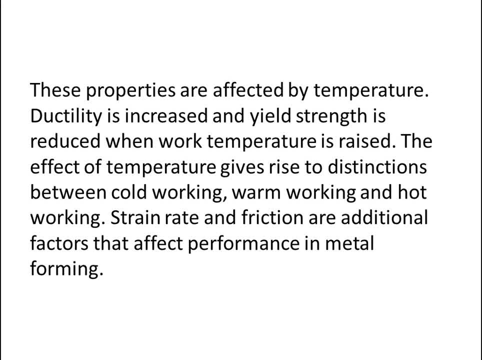 increased and early strength is reduced and work temperature is raised. so ductility is proportional to temperature and early strength is inversely proportional to temperature. the effect of temperature gives rise to distinctions between cold working, warm working and hot working. stress, strain rate and friction are additional factors that affect performance in metal forming.